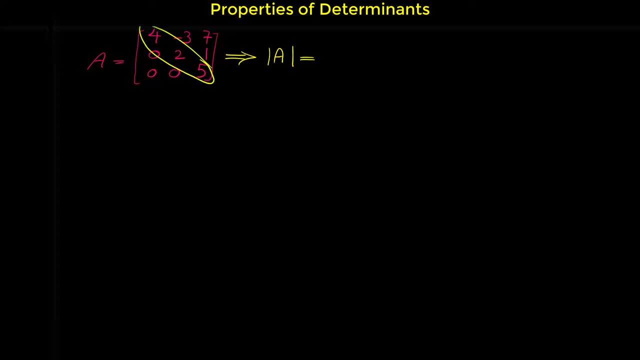 product of the elements of the main diagonal. So you don't need to use the regular formula of the determinant of the matrix. Simply multiply these elements and that is the determinant of the matrix. so determinant of the matrix a is 4 times 2 times 5. 4 times 2 is 8, 8 times. 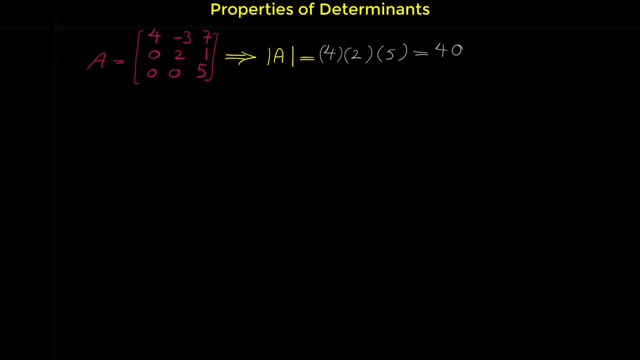 5 is 40. so determinant of this matrix is 40. let me show you another example. consider this matrix. matrix B is 7 0 0 0. 5 0 0 0 negative 1. this is a diagonal matrix because only the elements of the main diagonal are nonzero and the all. 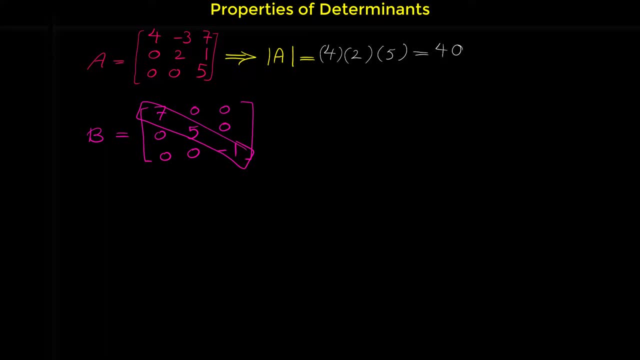 the elements above the main diagonal and below the diagonal are 0, so this is a diagonal matrix, so this is a diagonal matrix and so determinant of this matrix, determinant of the matrix B, is the product of these elements 7 times, 5 times negative, 1, which equals negative. 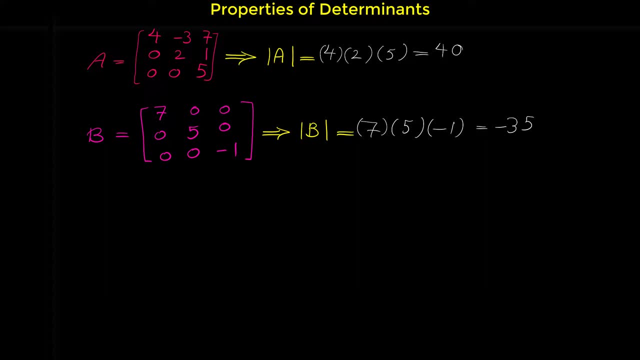 35. let me show you an example of a lower triangular matrix. consider this: 4 by 4 matrix: 1, 0, 0, 0 negative. you say Z signal. if you have this matrix, say plus 1, you answer, and below this you say thisquier, you just put their. 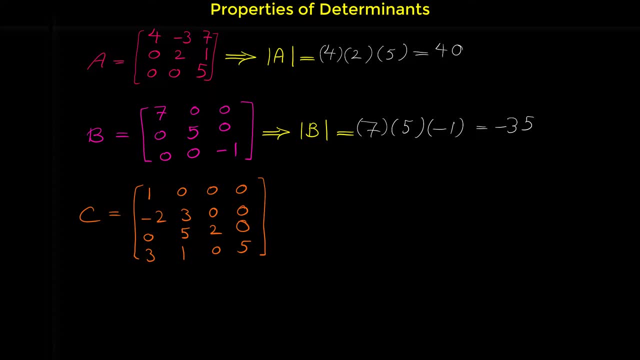 if either of them is égal to a negativeidade, then you are performing better. if so, then I want to make sure you know that I am making sure you answer exactly other than以上. perhaps I don't like giving no alpha K는. Let's say negative 2, 3, 0, 0, zero, 2 and the 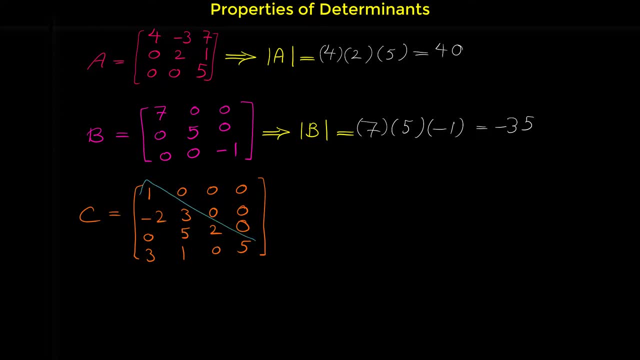 last row is the common king if this is a lower triangular matrix, because all the elements above the main diagonal, the main diagonal is this row perspective. so you see that. and the last row is the common king if this is a lower triangular matrix, because all the elements above the main diagonal, the main diagonal is this row perspective. so you see that. 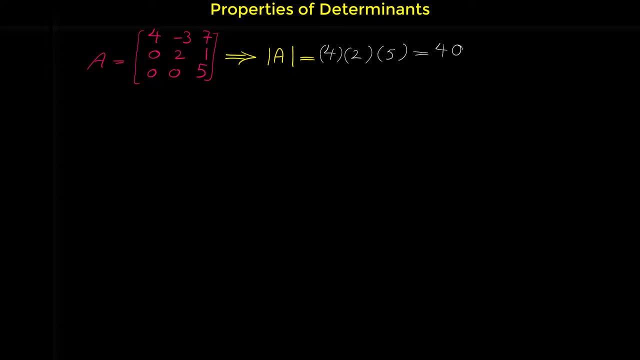 so determinant of this matrix is 40.. let me show you another example. consider this matrix. matrix b is seven zero zero, zero, five, zero, zero, zero, negative one. this is a diagonal matrix, because only the elements of the main diagonal are nonzero and all the elements above the main diagonal and 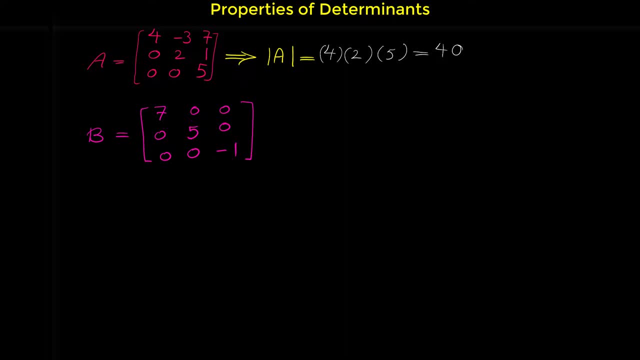 below the diagonal are 0. so this is a diagonal matrix and so determinant of this matrix. the of the matrix B is the product of these elements 7 times 5 times negative 1, which equals negative 35. let me show you an example of a lower triangular matrix. 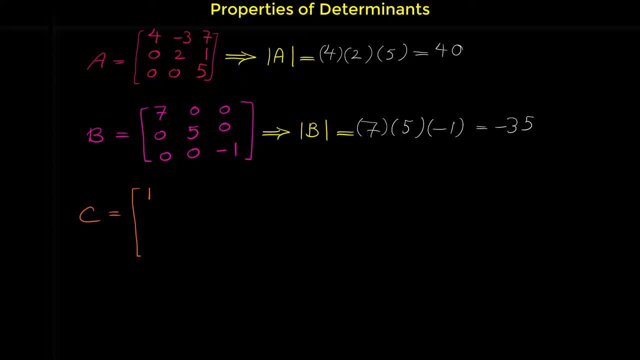 consider this four by four matrix: one zero zero, zero, negative, two, three zero zero, zero, five, two, and the last row is three. one zero, five, for example, this is lower triangular matrix, because all the elements above the main diagonal, the main diagonal is this: one, three, two, five, all the. 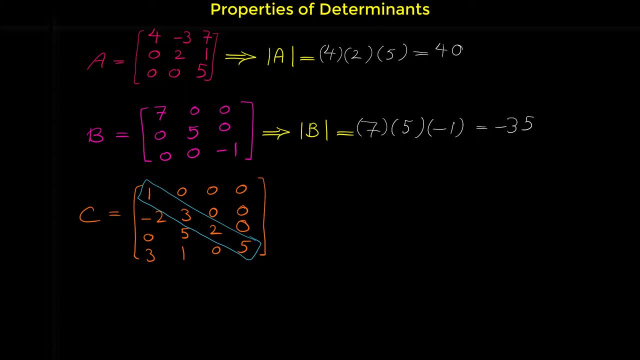 elements above the main diagonal are zero. so this is a large triangular matrix and the determinant of this matrix, determinant of the matrix c, is one times three times two times five. one times three is three. three times two is six. six times five is thirty. this is how you can find the determinant of. 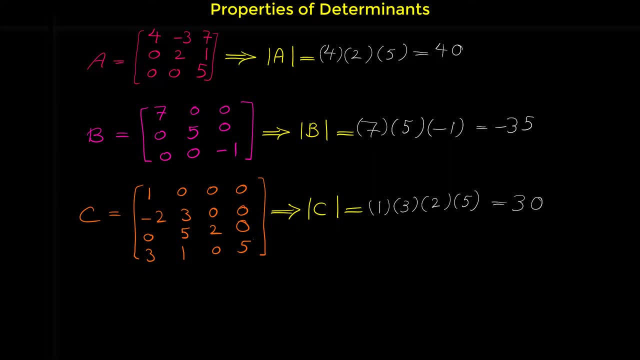 upper triangular, large triangular or diagonal matrices simply multiply the elements of the main diagonal. the next property we want to learn here is that if we transpose a matrix, determinant of the matrix doesn't change. so the next property is that if we have a matrix, say a determinant of the matrix a is equal to 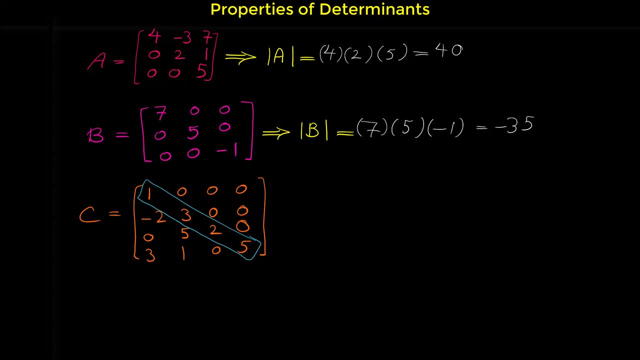 this one, three, two, five, all the elements above the main diagonal are zero. so this is a large triangular matrix and the terminal of this matrix, the terminal of the matrix c, is one times three times two times five. one times three is three. three times two is six. six times five is: 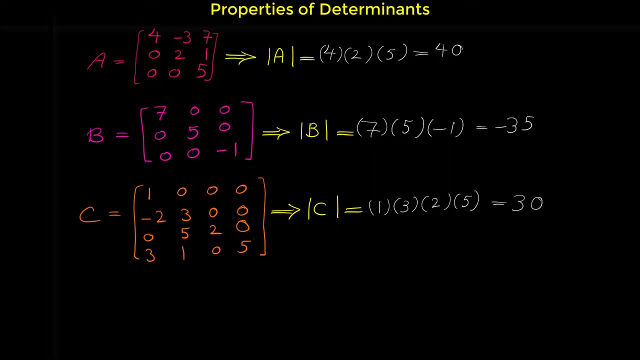 30.. this is how you can find the terminal of upper triangular, large triangular or diagonal matrices: simply multiply the elements of the main diagonal. the next property that we want to learn here is that if we transpose a matrix, the terminal of the matrix doesn't change. 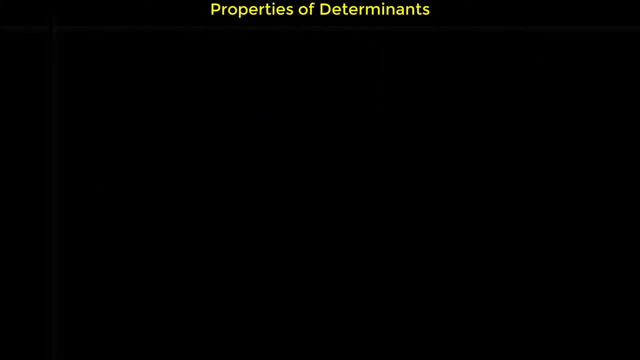 so the next property is that if we have a matrix, say a, the terminal and of the matrix a is equal to the determinant of the transpose of the matrix a. let me show you an example. let's try the 2 by 2. matrix 3: 1, 4, 5. the terminal of the matrix a is: 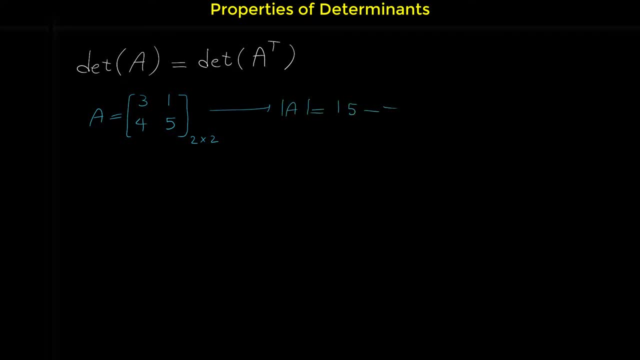 3 times 5, 15 1 times 4, 4. 15 minus 4 is 11.. we know how to find the terminal of a 2 by 2 matrix: 3 times 5 minus 1 times 4.. now let's find the transpose of this. 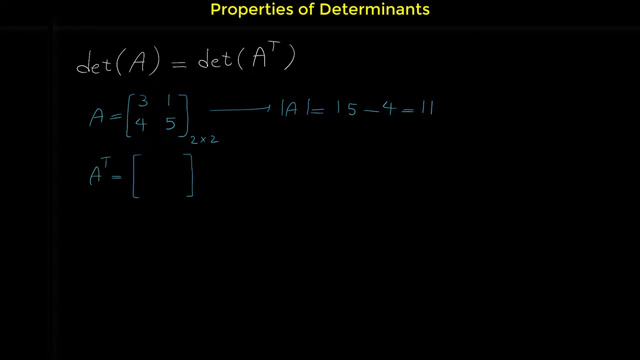 matrix. we know that for finding the transpose simply we have to make the rows columns in the transpose matrix. the rows of the original matrix are columns 3: 1 is the first row, so we make it the first column. the next row is four, five. we make it the next column, the terminal of. 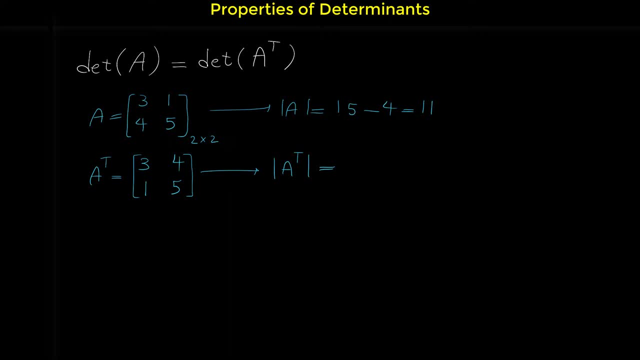 the matrix, the terminal of a transpose, is 3 times 5, 15, 1 times 4 or 4 times 1, is 4. 15 minus 4 is element. as you can see, these two numbers are the same. so when we transpose a matrix, the terminal. 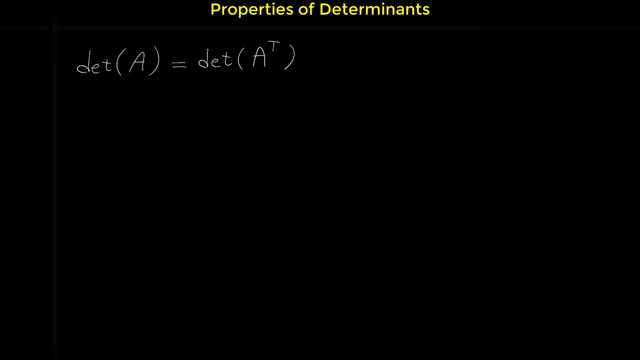 determinant of the transpose of the matrix a. let me show you an example. let's try the two by two matrix three, one, four, five. the determinant of the matrix a is three times five, fifteen, one times four, four. fifteen minus four is eleven. we know how to find the determinant of a two by two matrix. 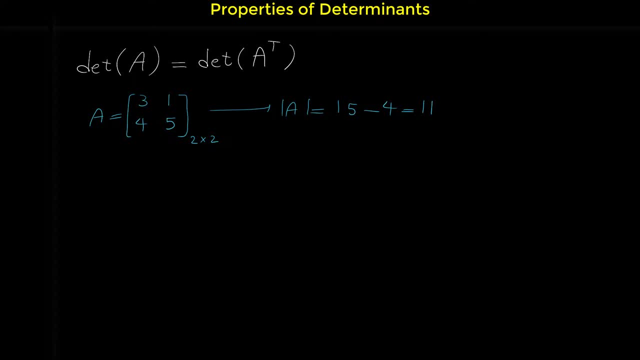 three times five minus one times four. now let's find the transpose of this matrix. we know that for finding the transpose, simply we have to make the rows columns in the transpose matrix. the rows of the original matrix are columns three. one is the first row, so we make it the first column. the next row is four, five, we make it the next column, the determinant. 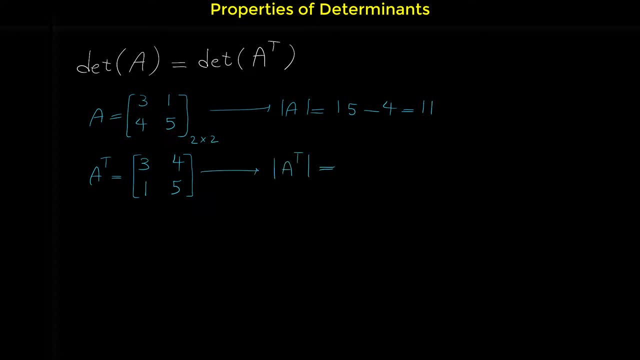 of this matrix, the determinant of a transpose is three times five, fifteen, one times four or four times one is four. fifteen minus four is element. as you can see, the following is a three, three and a six, two, a three and a half and three times one times and a half, or the next row is four, fifteen. 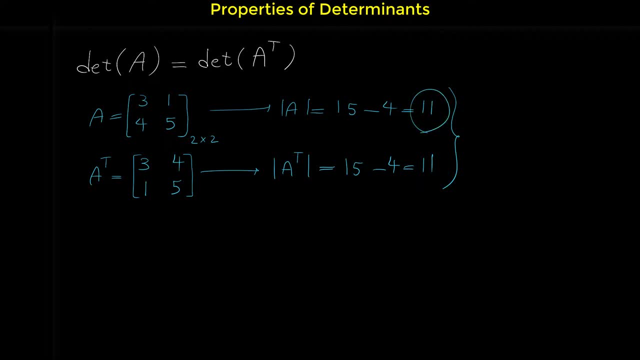 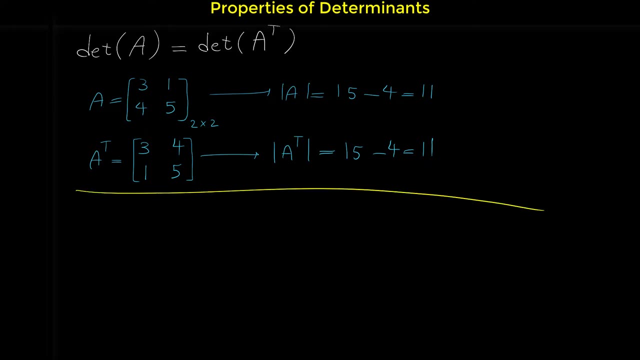 you can see, these two numbers are the same. so when we transpose a matrix, determinant doesn't change. the next property is that if we multiply two matrices by each other, a times b- determinant of a times b is equal to determinant of a times by determinant of the matrix. 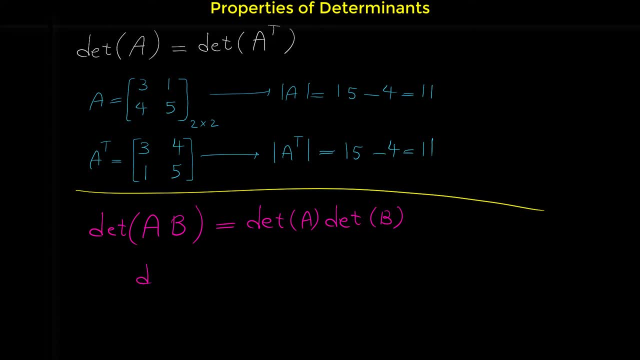 b. note that for sum or difference of two matrices we don't have such property. determinant of a plus b is not equal to the determinant of a plus the determinant of b. we don't have such property for the matrices in general and also the determinant of a minus b. 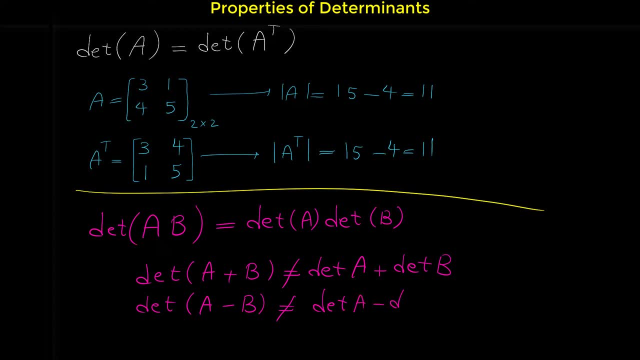 is not equal to the determinant of a minus the determinant of b. but if we multiply two matrices, say those matrices are a and b- determinant of a times b is equal to the determinant of a times y determinant of b. but for sum or difference of two matrices we don't have. 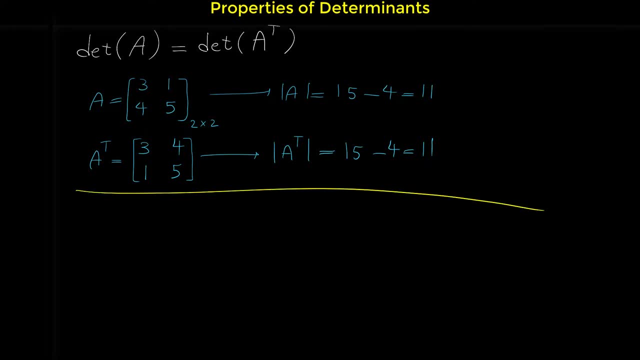 doesn't change. the next property is that if we multiply two matrices by each other- a times b- the of a times b is equal to determinant of a times by determinant of the matrix. note that for sum or difference of two matrices we don't have such property. 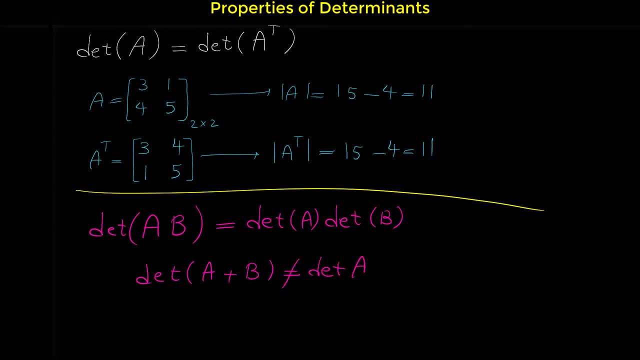 determinant of a plus b is not equal to the determinant of a plus the determinant of b. we don't have such property for the matrices in general. and also the determinant of a minus b is not equal to the determinant of a minus the determinant of b. but if we multiply two matrices, 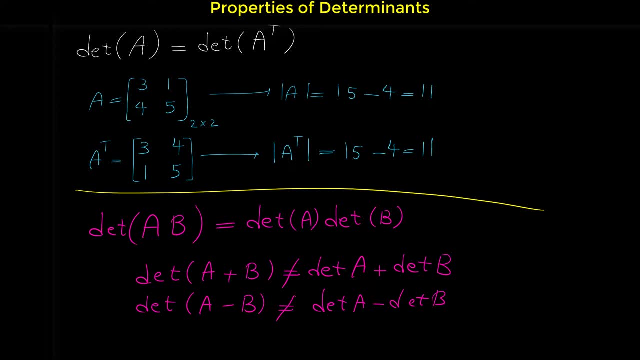 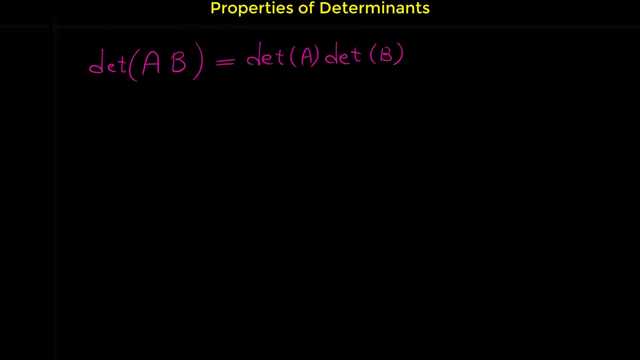 say those matrices are a and b. determinant of a times b is equal to the determinant of a times y determinant of b. but for sum or difference of two matrices we don't have such property. let me show you an example of this property. suppose matrix a is two, three negative one, five, and matrix b is seven, ten, five, seven. 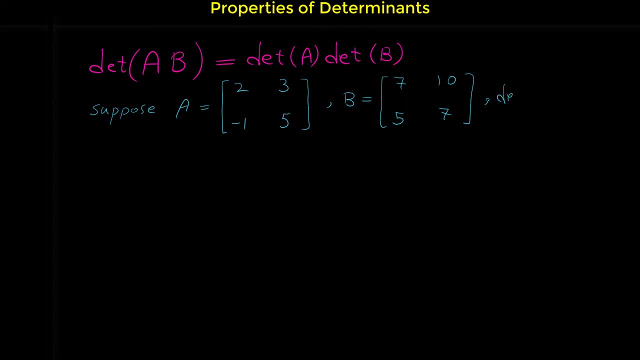 and we are asked to find determinant of a times b. for finding determinant of a b, first we can multiply the matrix a in the matrix b and then we can find determinant of that matrix. but multiplying two matrices, even for two by two matrices, is a bit hard. it needs a little. 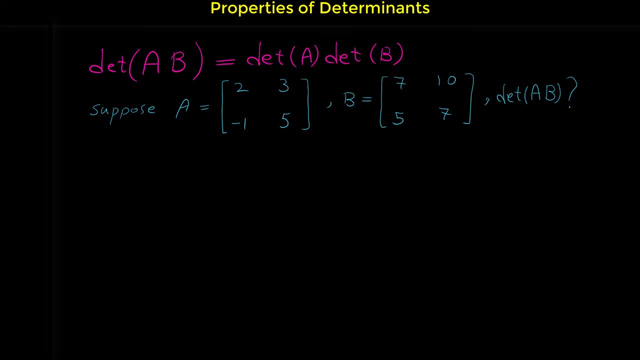 calculation. the easier way that we can find determinant of a times b is using the matrix b, this relation. we know that, in general, determinant of a- b is equal to determinant of a times determinant of b, and so, based on this, we can find simply determinant of a determinant of. 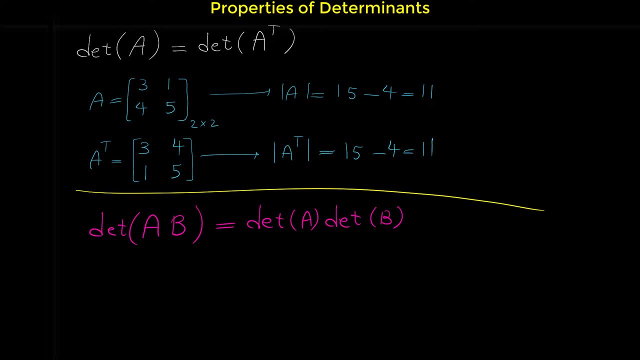 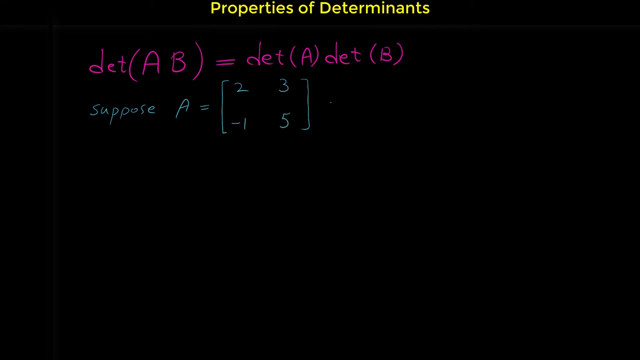 such property. let me show you an example of this property. suppose matrix a is 2, 3, negative 1, 5, and matrix b is 7, 10, 5, 7, and we are asked to find determinant of a times b. for finding determinant of a, b: 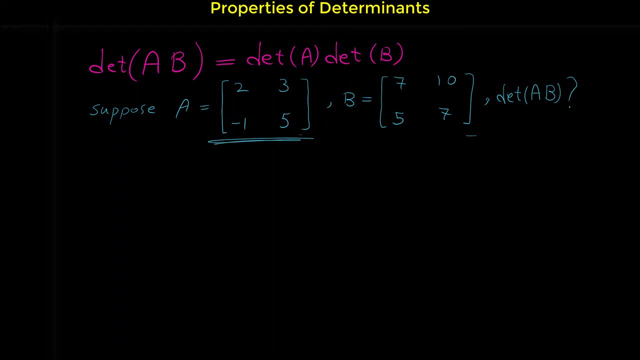 first we can multiply the matrix a in the matrix b and then we can find determinant of that matrix. but multiplying two matrices, even for two by two matrices, is a bit hard. it needs a little calculation. the easier way that we can find determinant of a times b is using this relation. 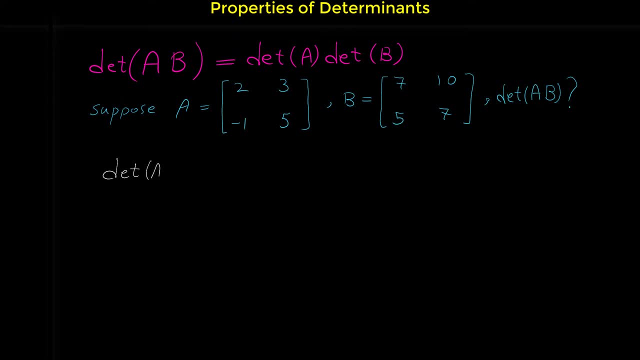 we know that, in general, determinant of a, b is equal to the determinant of a times the determinant of b, and so, based on this, we can find simply determinant of a determinant of b and then multiply those numbers by each other. what is the determinant of this matrix? two times five minus three times, so two times. 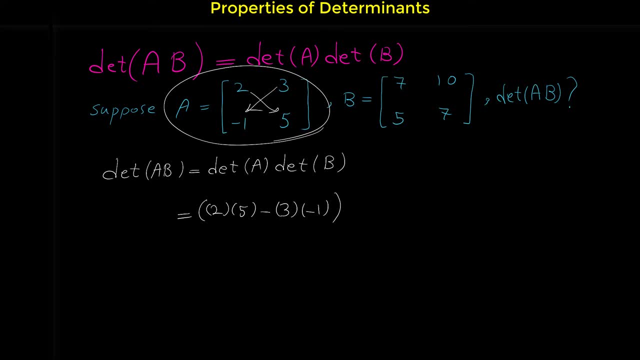 five minus three times negative one. we have to multiply this by determinant of the other ones: seven times seven minus ten times five. this equals 13, and the other one is negative. one plus 47 minus 50 is negative one, and this equals negative 30.. so, as you can see, you can use this relation for solving these type of questions. 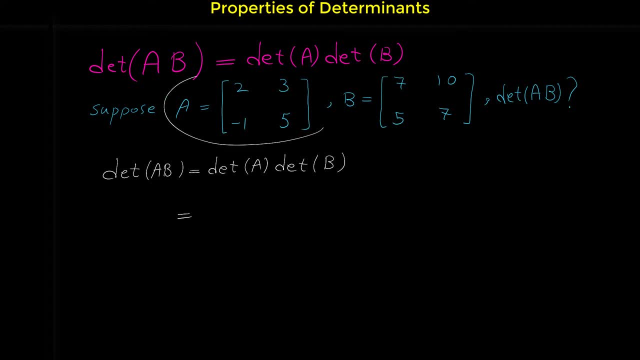 b and then multiply those numbers by each other. what is the determinant of this matrix? 2 times 5 minus 3 times. so 2 times 5 minus 3 times negative 1. we have to multiply this by determinant of the other one: 7 times 7 minus 10 times 5. this equals 13. and the other? 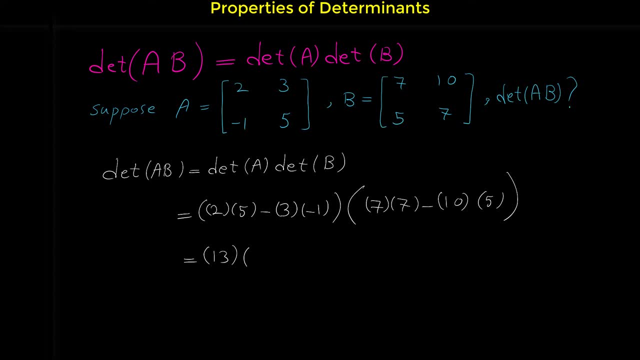 one is negative 1 plus 47 minus 50 is minus 2.. you can just use the numerator and the denominator to figure this out. now let's check the denominator multiple times: negative 1 and this equals negative 30.. so, as you can see, you can use this relation for solving. 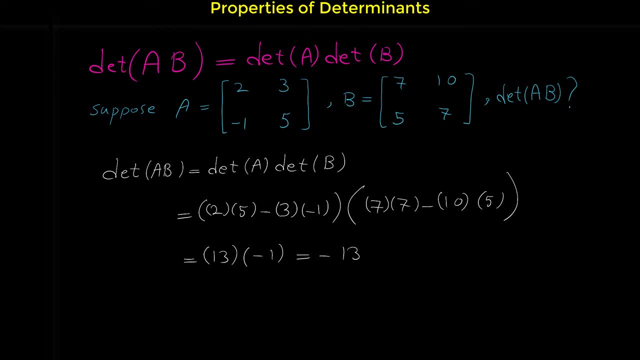 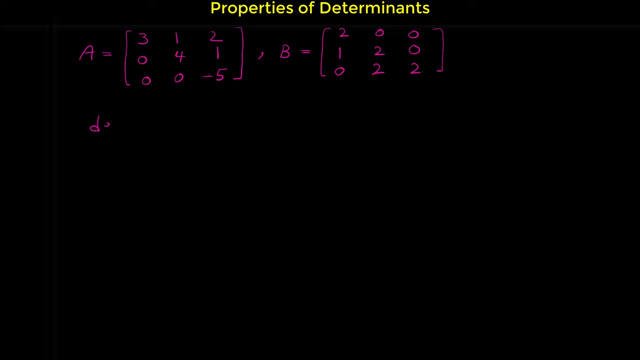 these type of questions. let me show you another example of this property. we are given matrix a, a, 3 by 3 matrix with these elements: 3, 1, 2, 0, 4, 1, 0, 0, negative 5, and the matrix b is 2, 0, 0, 1, 2, 0, 0, 2, 2 and we are asked to find determinant. 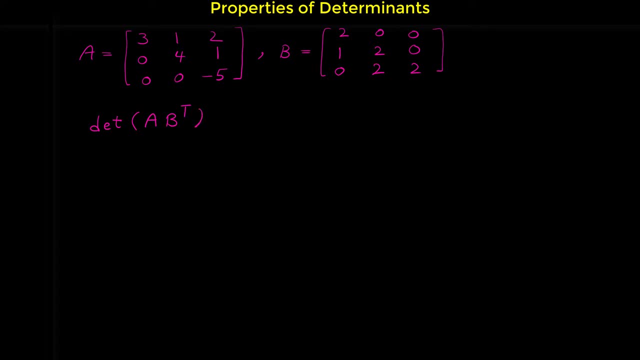 of a times b transpose. for finding determinant of a times b transpose, we can first transpose the matrix b to find b transpose and then we have to multiply a by the transpose of this matrix, which is a bit hard because it's a 3 by 3 matrix. 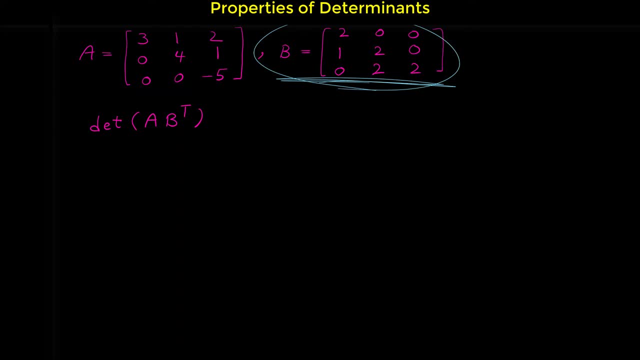 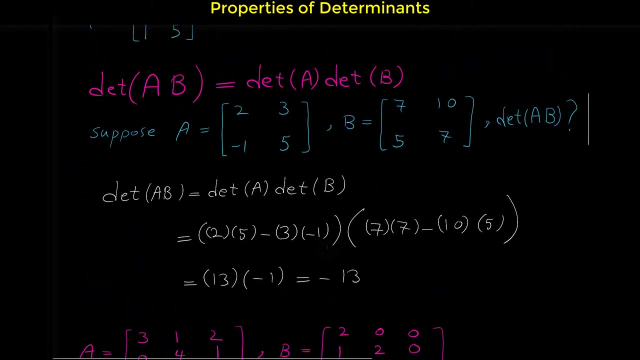 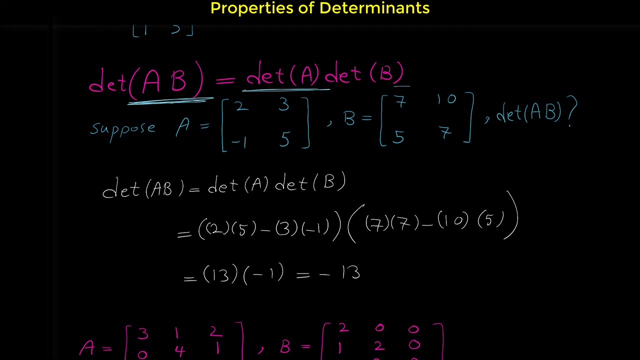 multiplied by another 3 by 3 matrix. it needs some calculations and then we can find the terminal of that matrix. the easier way is to use the above properties first. so based on the property that we learned here, determinant of the multiplication, the product of two matrices is equal to determinant of the first matrix times by determinant of the other. 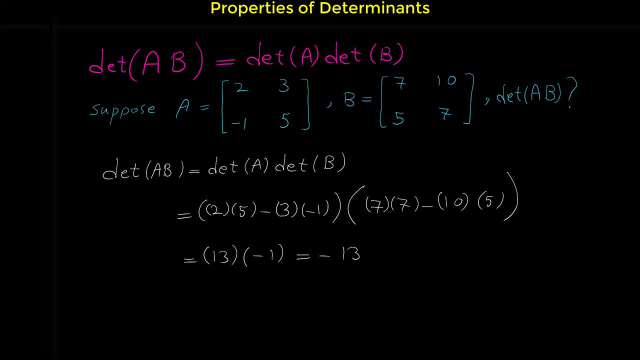 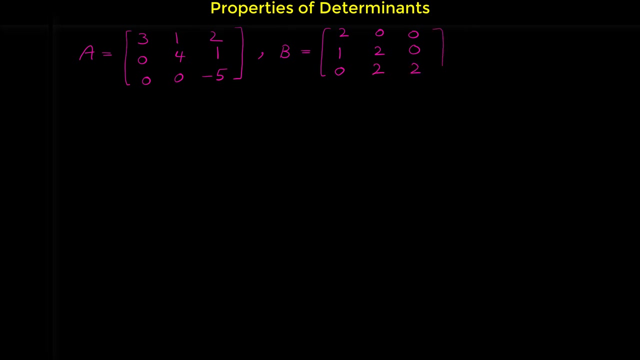 let me show you another example of this property. we are given matrix a a, three by three matrix with these elements: three, one, two zero four, one zero zero, negative, five. and the matrix b is two zero zero one, two zero zero, two, two. and we are asked to find determinant of a times b transpose. for finding determinant of a times b transpose: 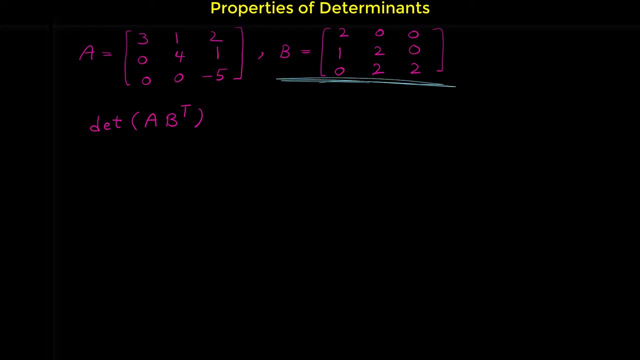 we can first transpose the matrix b to find b transpose and then we have to multiply a by the transpose of this matrix, which is a bit hard because it's a three by three matrix- multiply by another three by three matrix. it needs some calculations and then we can find the determinant of that matrix the easier way. 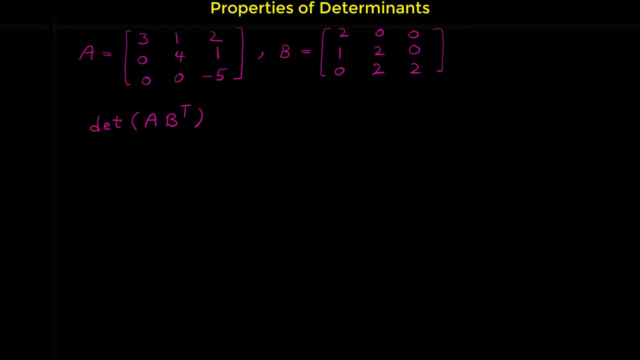 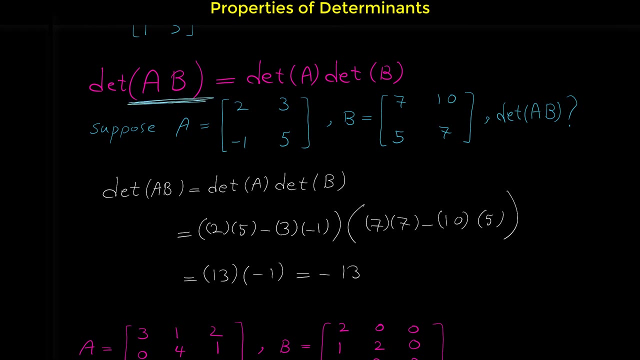 is to use the above properties first based on the property that we first, based on the property that we learned here, the determinant of the multiplication, the product of two matrices, is equal to determinant of the first matrix times by determinant of the other matrix. based on this property, we can say that we can find each one of them based on the new properties in group. 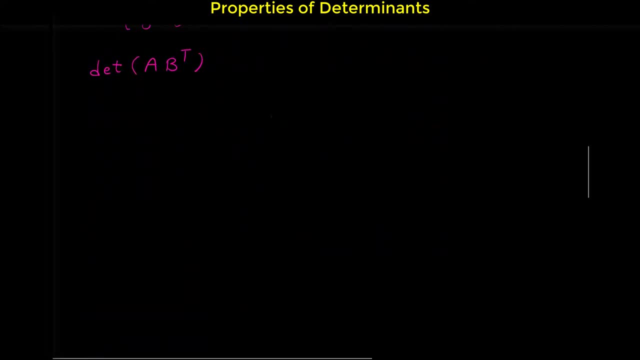 and I would say that we will always longtime that first property has the same value legally. for the next property we can say that determinant of a times b transpose equals to determinant of the first matrix a times y, determinant of the second matrix, b transpose. but if you remember from the properties, 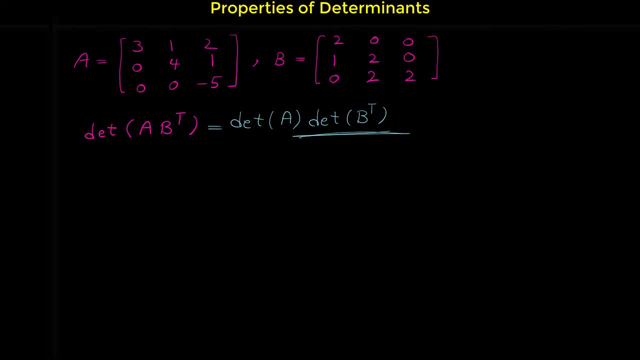 that we learned in this video: determinant of transpose of a matrix. determinant of this matrix. the transpose of this matrix is equal to the determinant of the original matrix. determinant of b- transpose is equal to determinant of b, so you don't need to even transpose this matrix. find determinant of matrix b and determinant of b- transpose is the same number. we learned this.